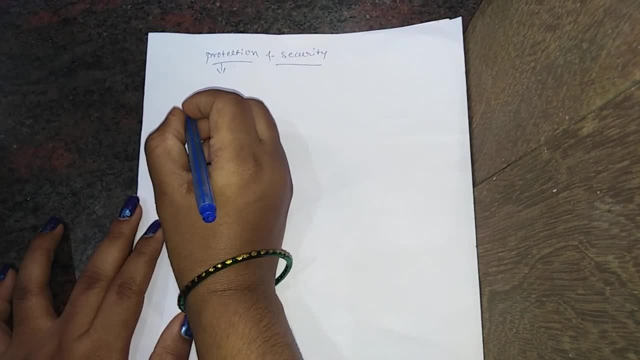 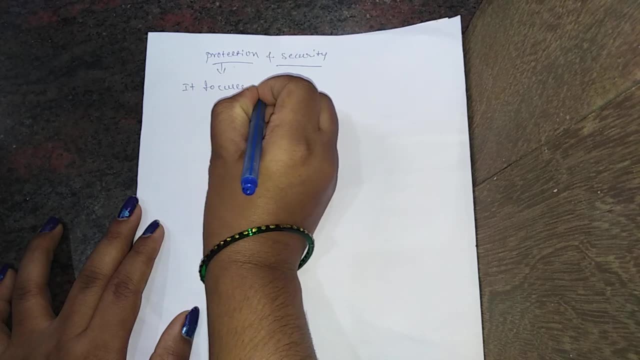 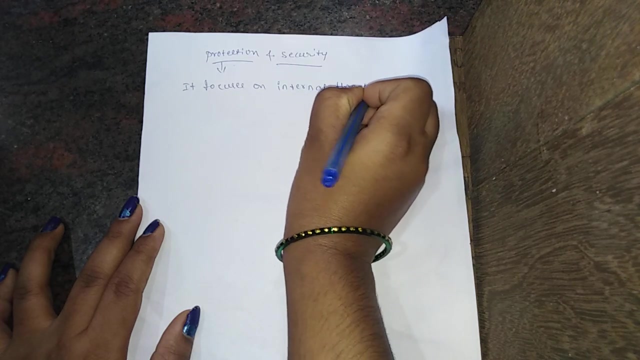 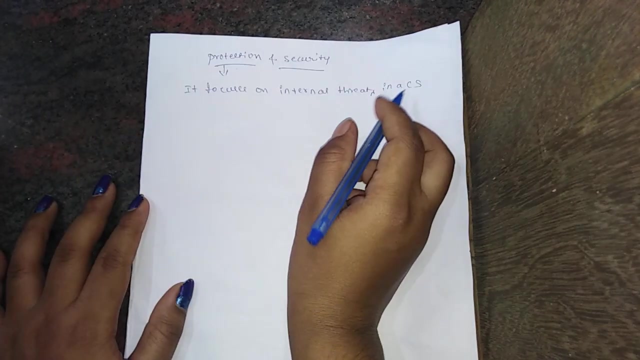 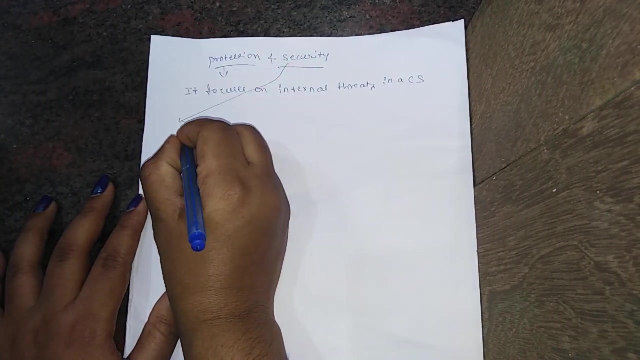 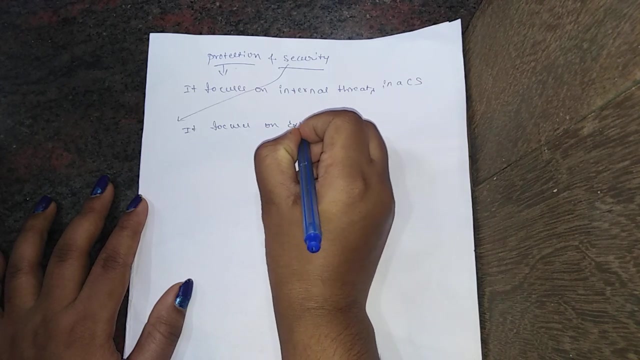 Security. Protection means it focus on the. it focuses on internal threat, Internal threats. That one threats in a computer system, Computer system. That one we can call it as a protection. Security means it focus on. it focuses on external threats in a computer. That one we can call it as a security. 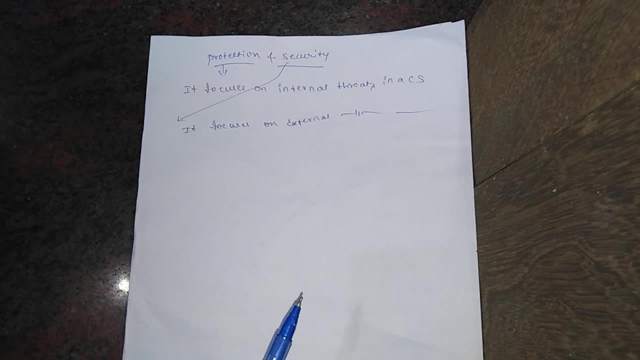 Do you know what is protection and what is security? What is the difference between protection and security? What is protection? Protection, It is focus on the internal threats, Internal threats in a computer system. Security means the focus on the external threats in a computer system. 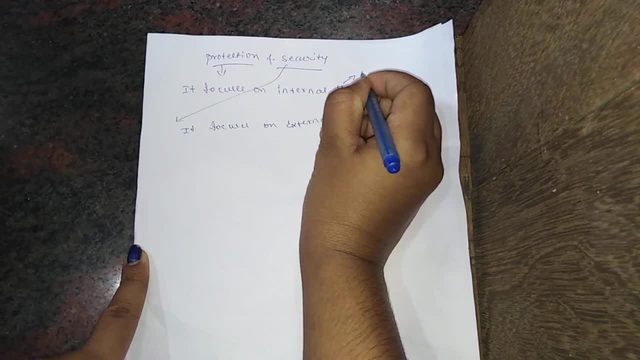 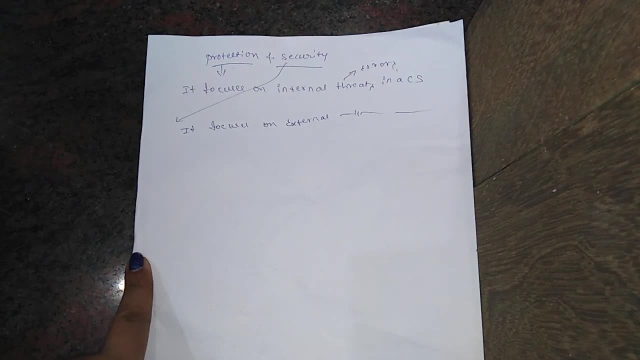 Threats means errors. Threats means errors or attackers- Errors or attackers In our protection and security. it interfaces. the resource utilization Is a very serious threat in a operating system. What is the resource? What are the resources we can use? 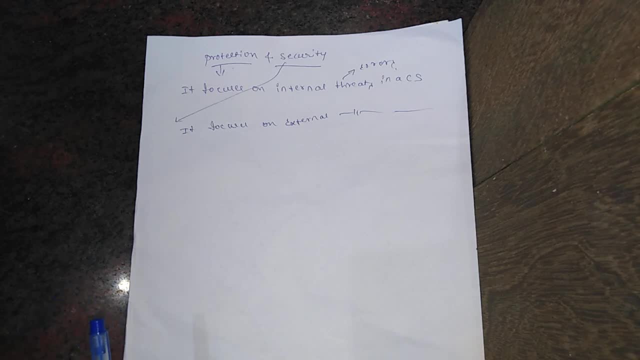 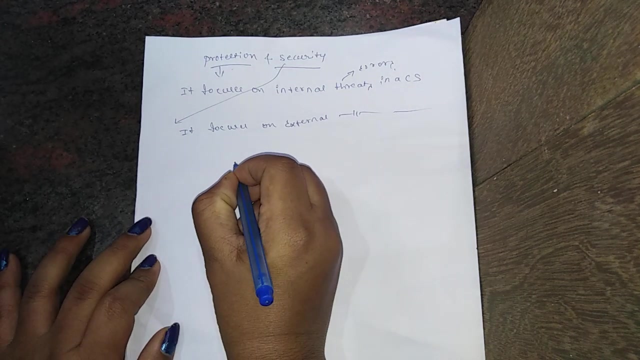 The natural of the threat depends on the natural of the resources. The manner in it is used. Threats means error. It will be depends on the natural of resources, What types of resources we can use. Resources File is the one. resources. 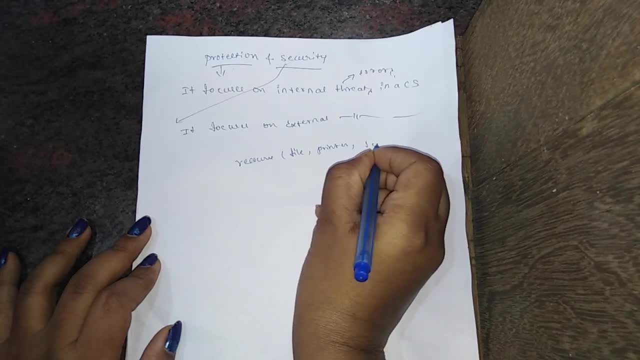 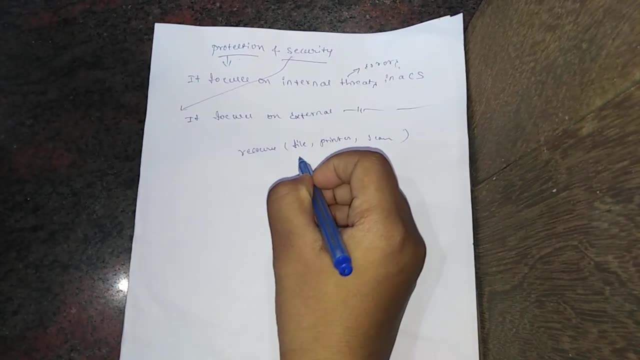 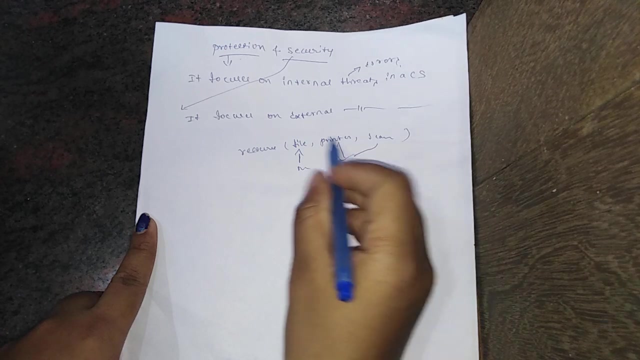 Error. Sometimes we can use the printer scanner. That is the resources we can use. File. This one we can call it as a protection. We can give a protection. this one, This one, we can give a security, Why? Because this one is the internal. 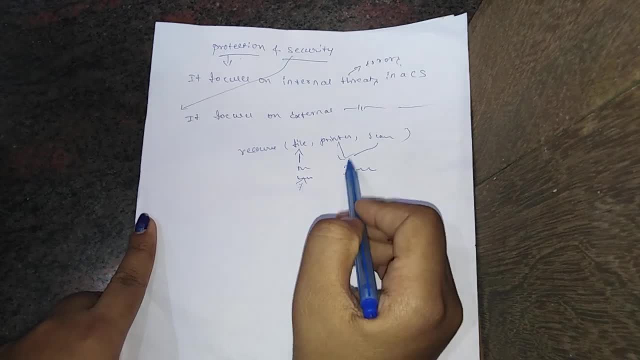 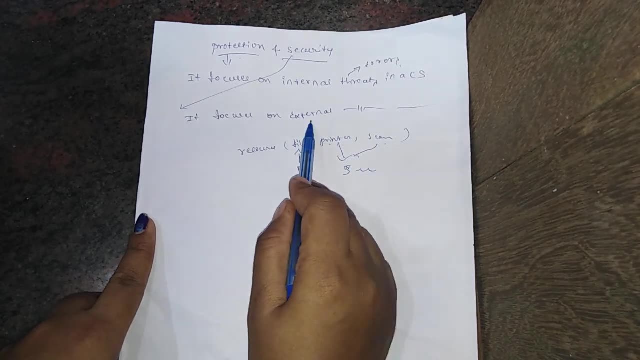 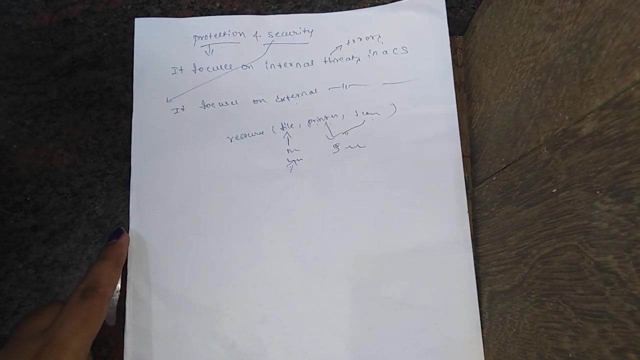 We can store the information in internal, This one we can protect or we can give a security to the this resources. This one is the external threats, Then anywhere operating system used to set of technique. of the computer threats Mainly, first one is the protection, Second one is the security: Protection and the security. 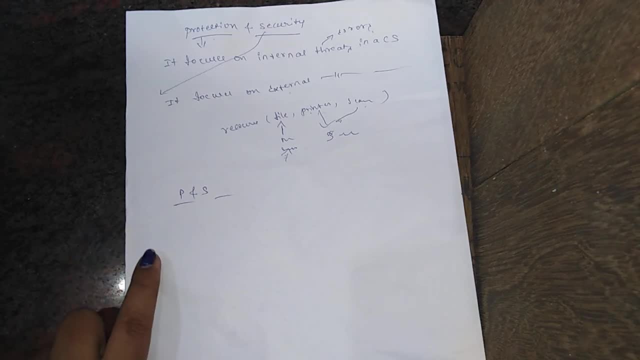 It involves protection. It means it involves the guarding a user data under the program against the interface by the other authorized user of the system. It means entry of the document It should protect is needed for the files under the computer. That one we can call it as a protection. 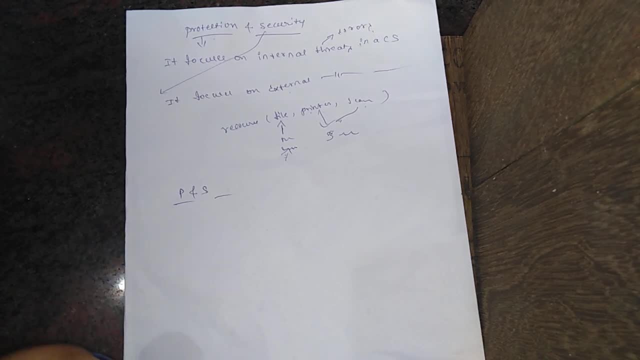 Security means It involves the guarding of the user data on the program against interface by the external entity. It means unauthorized person will be access the data. That type of threats we can occur means that one we can give a security. Then entity: entry of document. It should be protection file, computer documents. 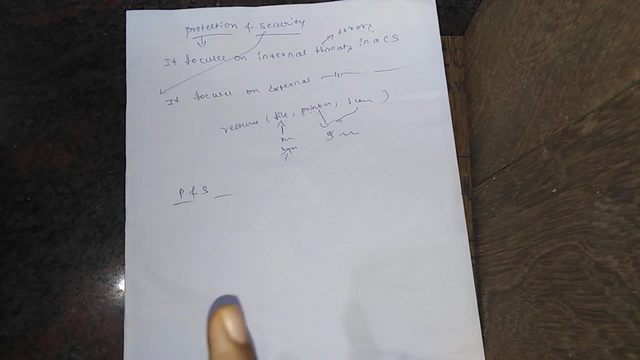 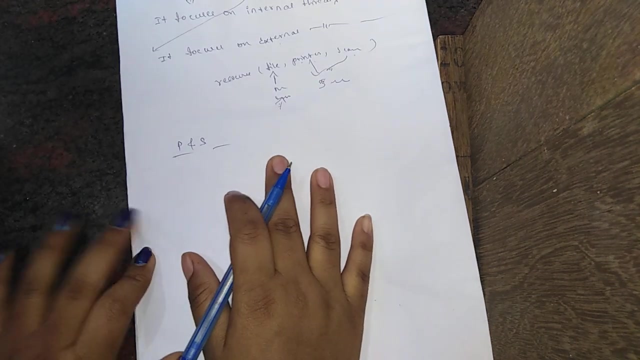 That one we can call it as a protection, Protection we can give to the internal threats. You know already what is the difference between protection and the security. Anywhere, two factor of protection will be there. Two protection will be there. First one is the security and the privacy. 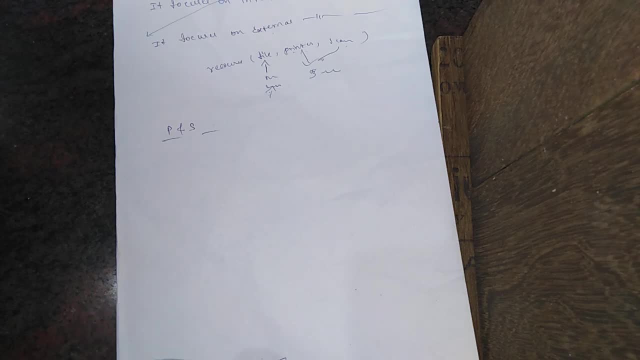 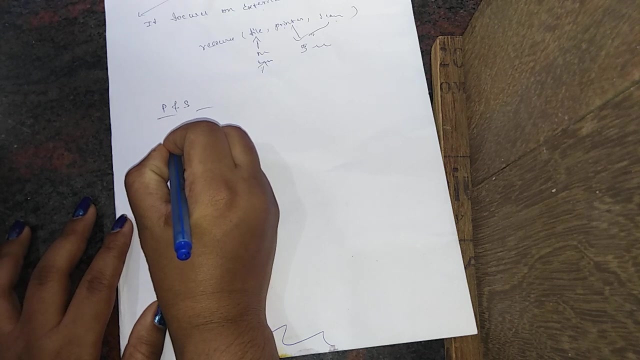 What is security? It implies that only the authorized user should be able to access the information. That one we can call it as a secrecy Or secret, we can given. We can give the security or give the secret. we can maintain. That one we can call it as a secrecy. 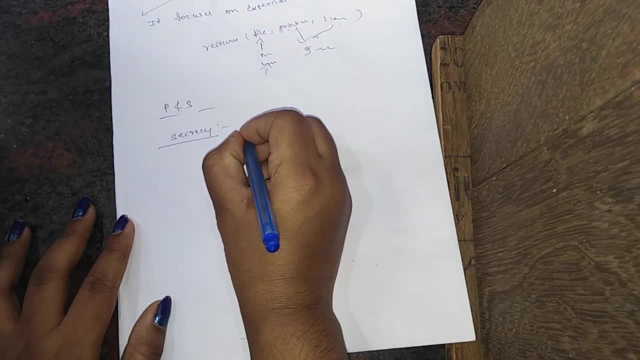 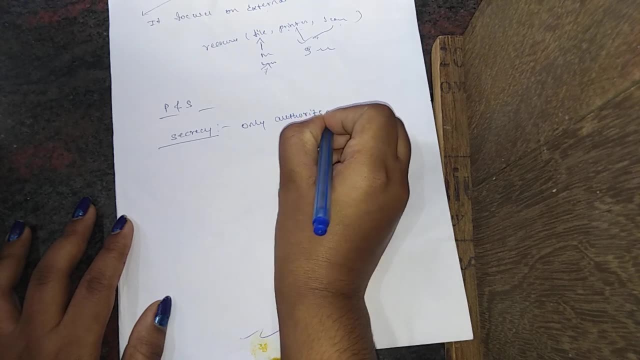 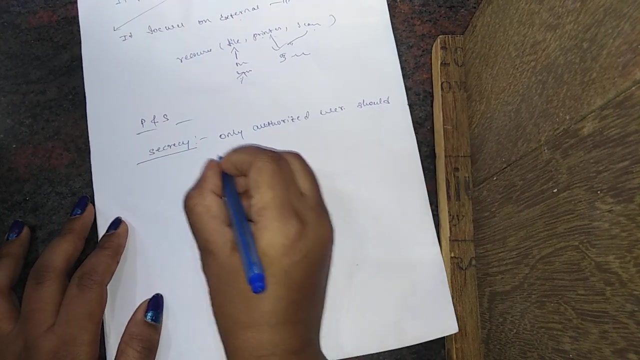 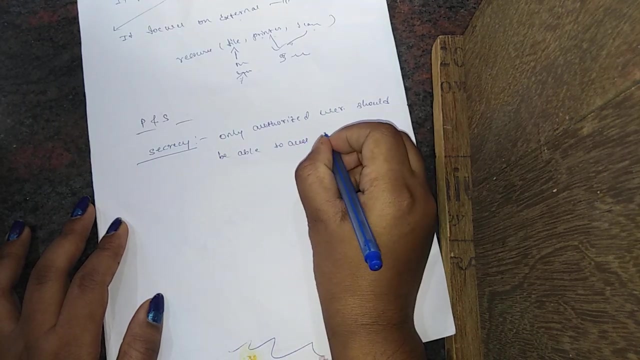 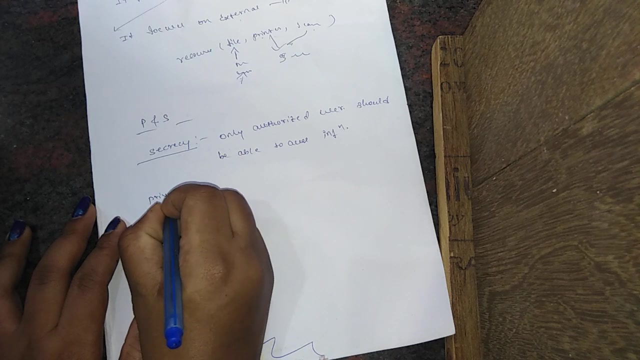 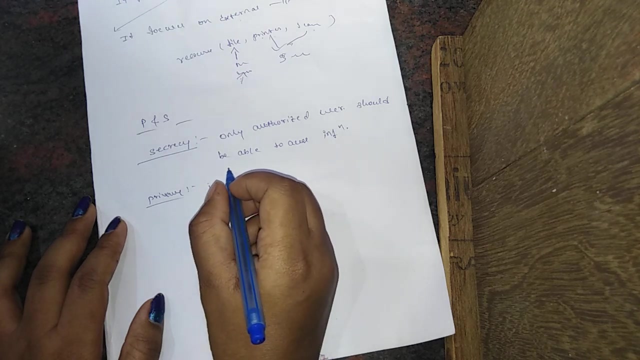 Secrecy means It implies that only authorized user should be able to access the information, That one we can call it as a secrecy. Then privacy means It implies the information It should only for the purpose Or intended. or what are the shared information? 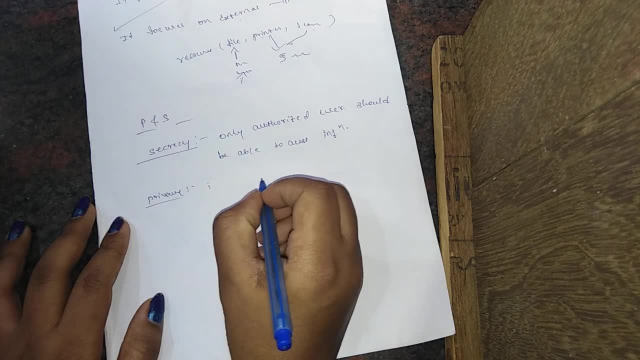 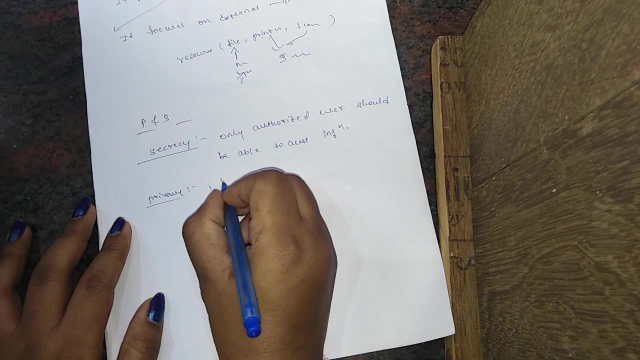 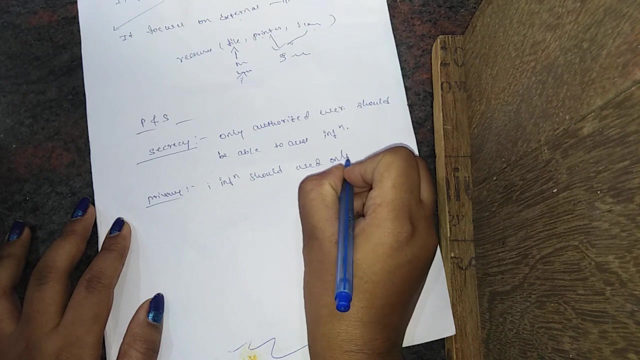 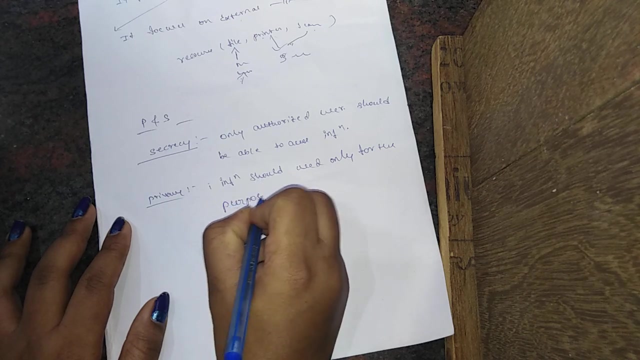 That one we can call it as a privacy. Privacy means information should used only for the purpose. Information Should Used only for the purpose Purpose. That one we can call it as the privacy. Anywhere authorized means What is authorized. 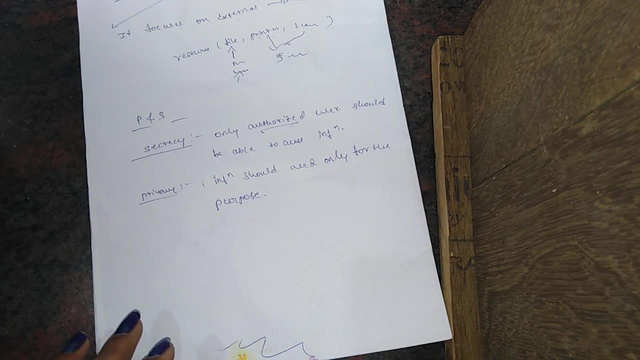 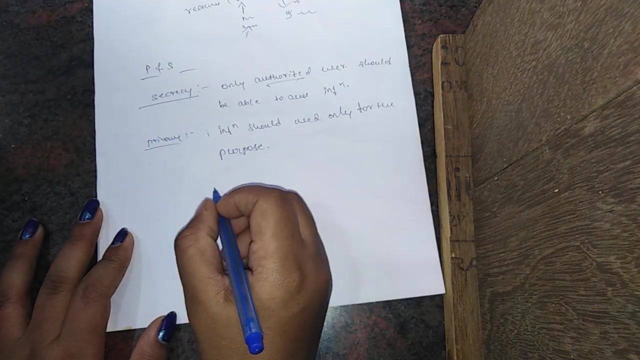 Or what is authentication? Authentication is the reasonable assurance, assurance that anyone will be access the information or who will be attempt to access the system or network. that one we can call it as a authorization or authorized person. we can call how we can. uh three mechanism: we can find out the these people is authorized or not. 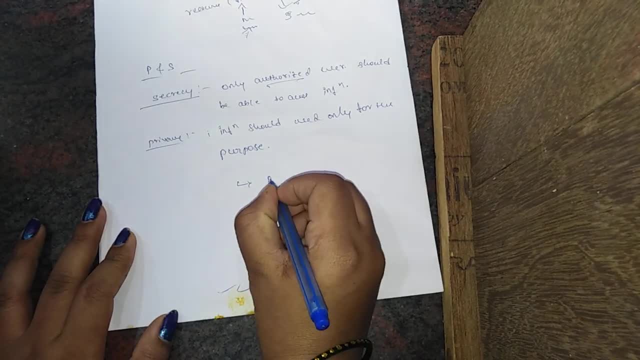 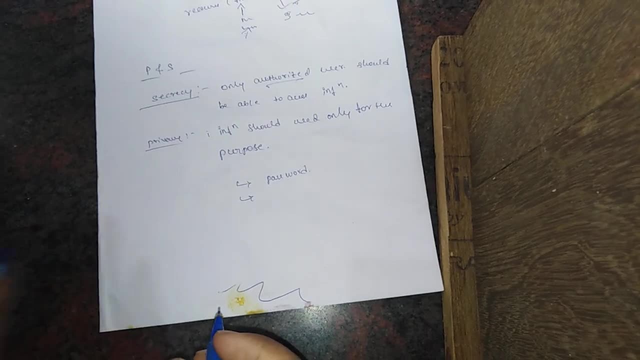 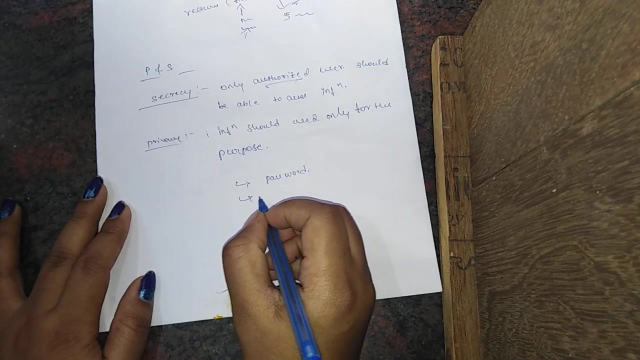 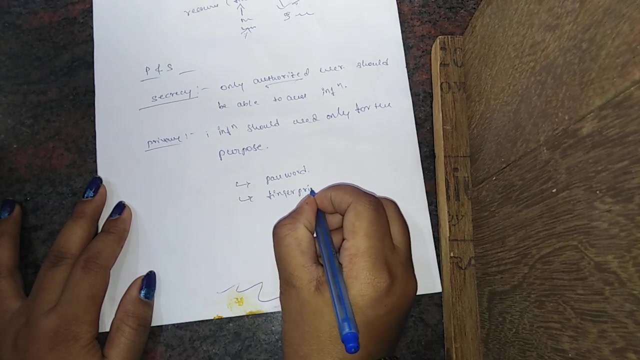 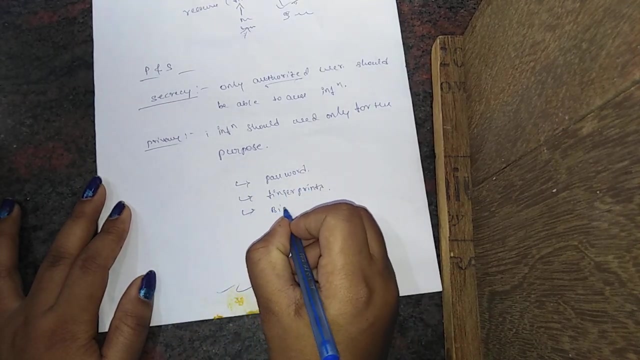 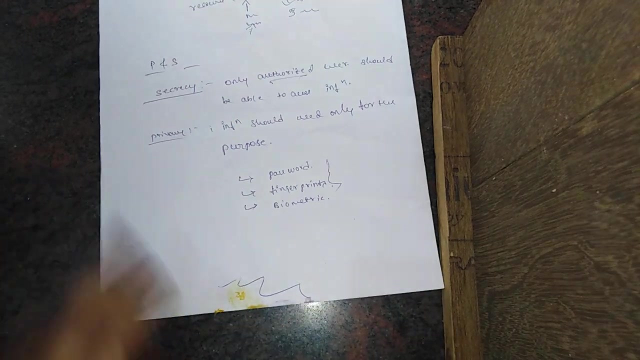 uh, what are the mechanism we can use? we can set the password. who will know the password? they will authorized, sometimes physical token, it means artifact, it means fingerprint, finger print friends, it match means that one also authorized person. then biometric, biometric, this one also authorizing person we knows means we can. 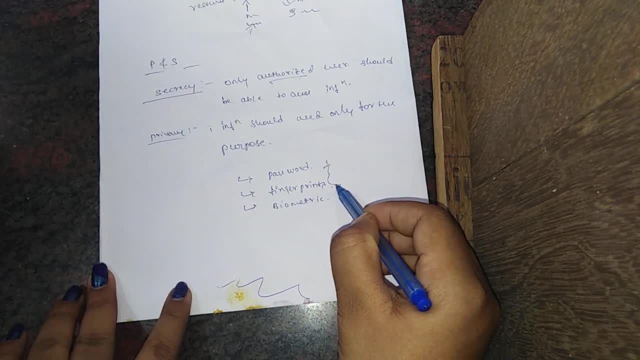 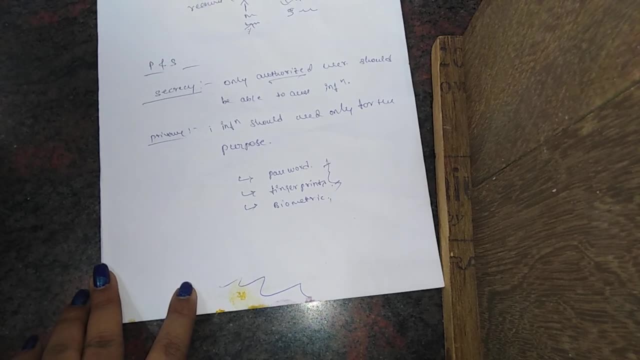 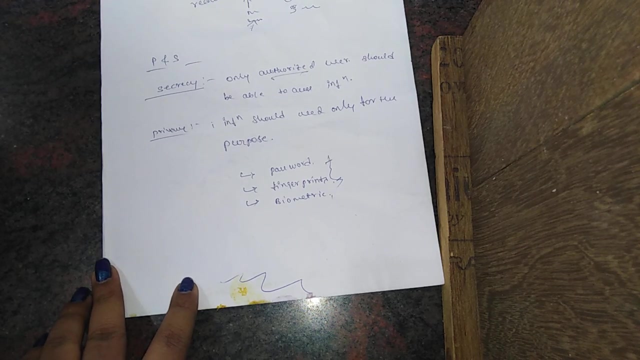 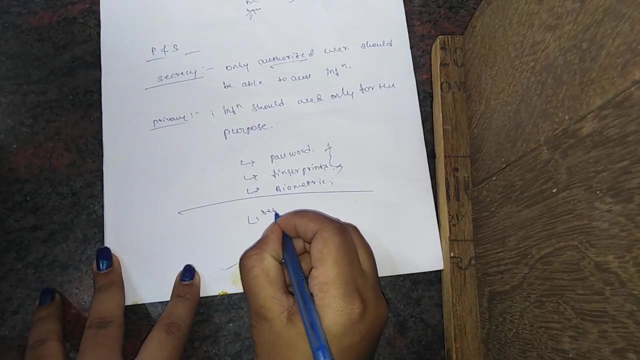 know the password. we can. we can give the fingerprint means it will be taken. biometrics means it will be taken. that day is we can protect or we can authorize a person. next, security attributes. what are the security attributes we can see? first one is security attributes. what are the security attributes will be there? first one is confidentiality. 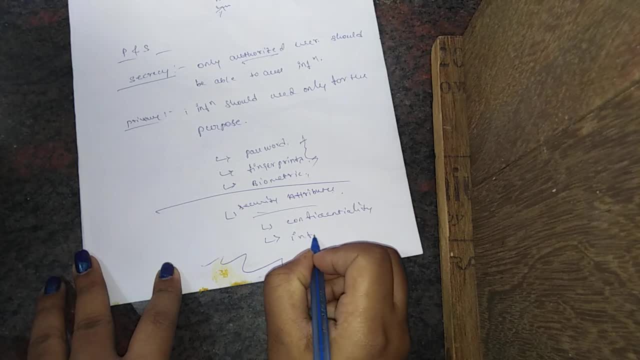 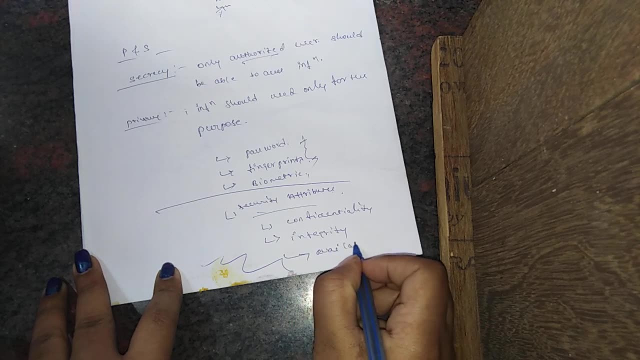 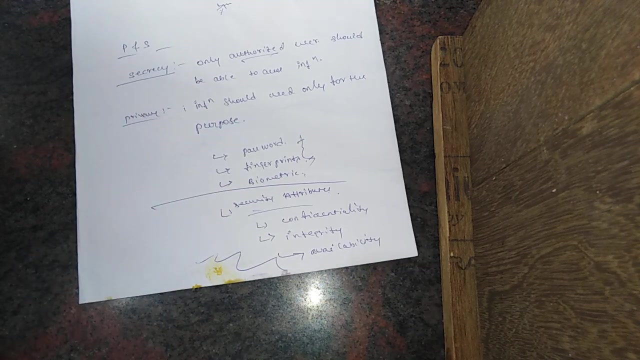 confidentiality. second one is integrity. last one is availability. availability: what is confidentiality? confidentiality is the prevention of authorized and modification of information resources. that one we can call it as a confidentiality. integrity means it is the prevention of authorized. it is the prevention of authorized, that one we can call it as an integration. 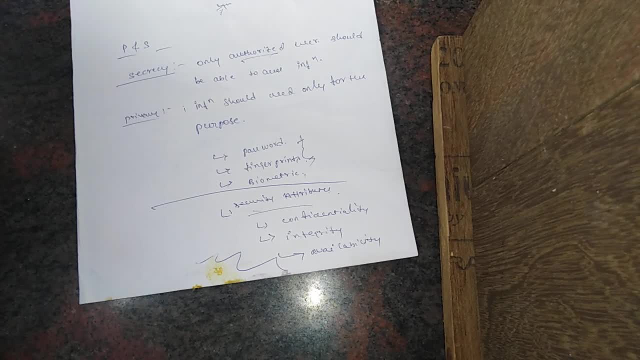 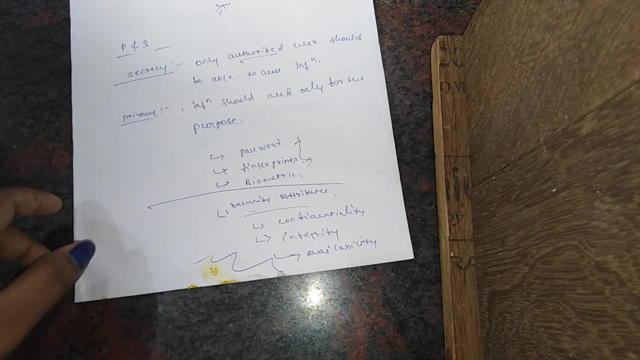 availability. it is the prevention of unauthorized withholding that the information, our resources, that one can call it as a availability. unauthorized user withholding the information or resources that one we can call it as availability in your security threats there are two times: direct and indirect. direct means we can directly, we can go andrhate and go fix service. 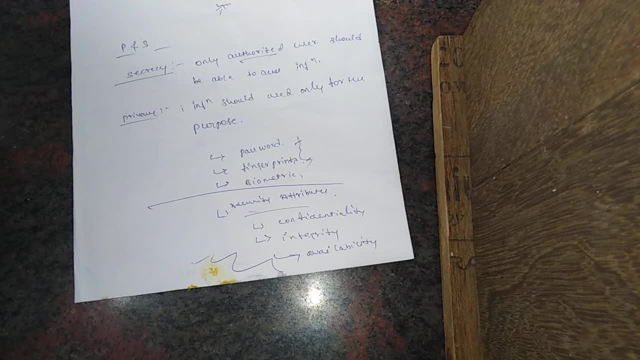 and what is the one we do to get natural and calibrated tools and features? we are. давайте sempre vega share this as an avaliability, which is our in user name us. our in user name, us. we are in his network, a recognized search group. it's called field control instance. 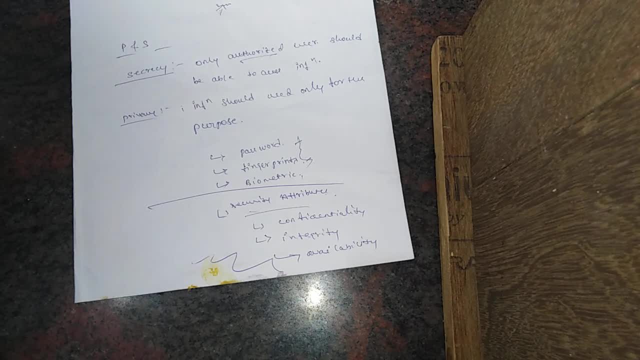 which holds the information that we are affected by Damn away, then recovery approaches are allowed to visit and bring to us hunting for information. we can do it again and also go and further along: forcat attack the specific system or whether from the outside attacker, hacker, from the. 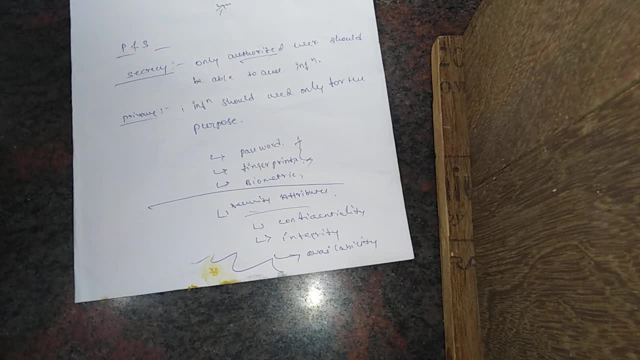 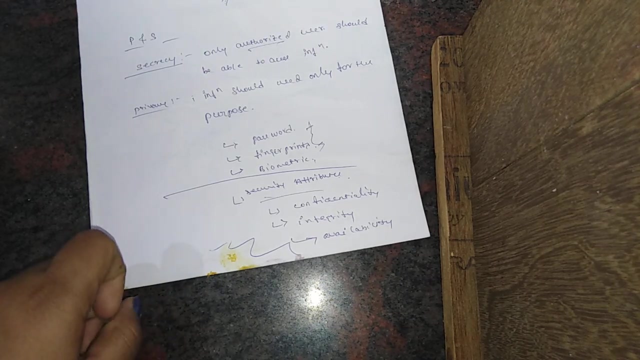 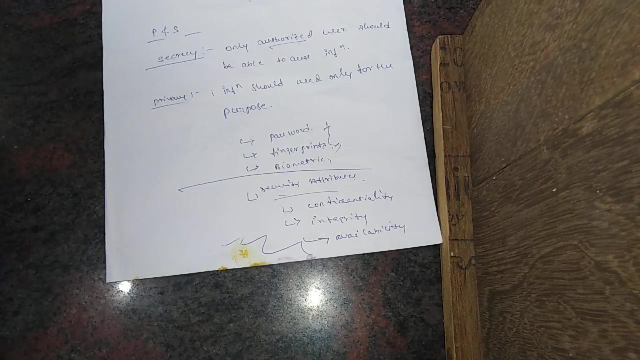 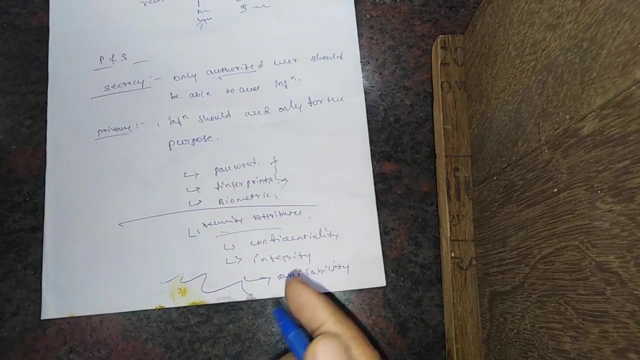 inside information- that one we can call it as a direct, indirect means, the general random attack must be commonly computer, whereas computer worms- that one we can call it as indirect attacks- in reason for taking security measurement, how, how we can prevent the information or prevent the resources means we can prevent the loss of data, we can prevent what, the reason we